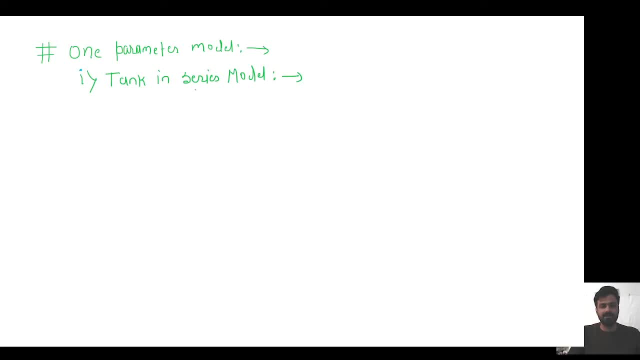 Okay, So in this here tank and series model is used for analyze the behavior of PFR. So here you can write: it is used to analyze the behavior of PFR. Okay, So I mean directly. you can write: the parameter will be number of tanks. It's very. 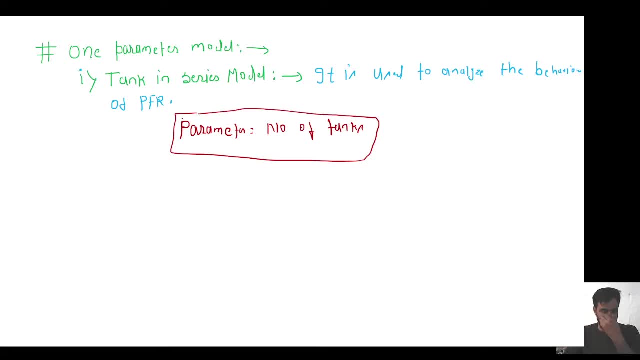 important that you need to understand here. the parameter will be number of tanks. Okay, So now I'm considering that And a number of history are connected in three. After that I will let you know the objective of these things. just try to understand the thing here. that is this year. 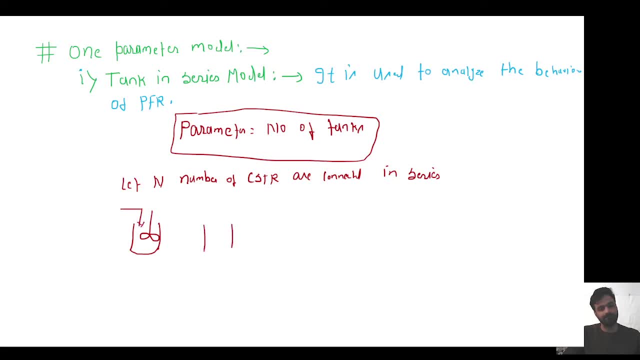 Is there any? Palmer and all the CSTR are connected over here is having same volume. okay, it is my assumption over here, because you know the thing becomes very easy. so the outlet, and again here it is real, again here it will be coming in this way again. 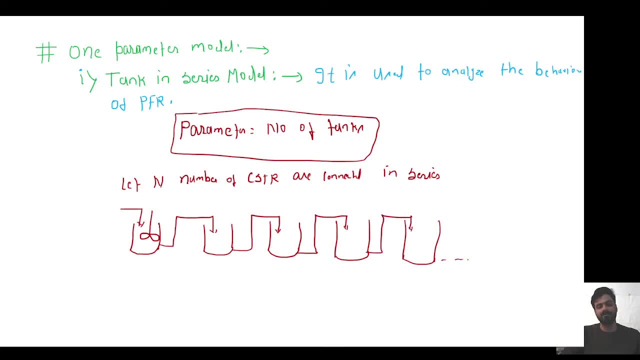 here it will be coming in this way again. here it will be coming and there is shown number of. I mean CSTR will be there and here it is outlet. okay, so CSTR is well known for the continuous stirring as well as uniform mixing. okay, so that's why there will be a stirrer over. 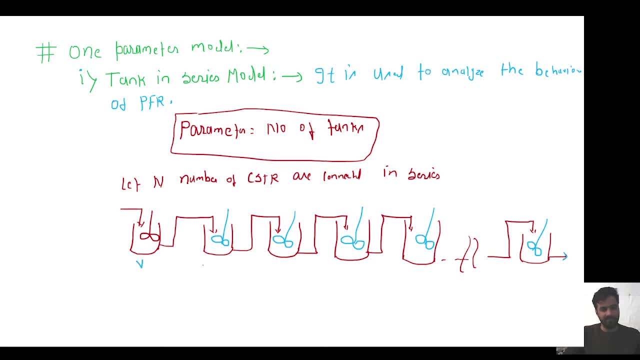 here. okay, now here I am assuming the volume of the CSTR is V, V, V, V, V and V. okay, and so here it will be: tau1, it equals to, tau2 is equals to, tau3 is equals to, and this equals to taun. so the it see dense time for al the CSTR. 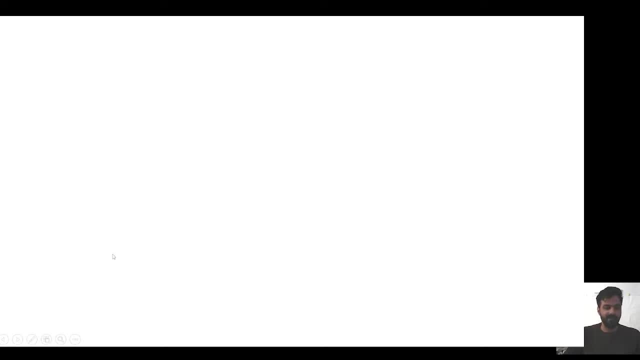 will be same. okay, next, my stand for one parameter. so for pulse stress and input will be applied for one one, one parameter. model pulse tracer experiment will be performed. ok, on the inlet of, on the inlet of CSTR. that is, you can say first, CSTR, are you getting next? so when we talk about my 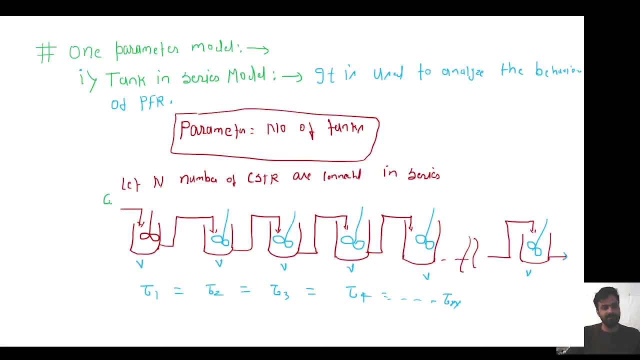 student here. here it is concentration. if you are assuming C naught, here concentration is C 1, here it will be C 2, here it will be C 3, here it will be C 4 and dot dot, here it will be C n. so what will? 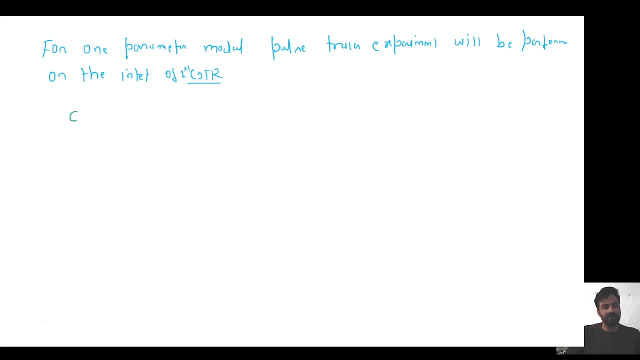 be the value of C 1 from here. so can I write C 1 that is equal to C 1 and C 2 that is equal to C 1 to C naught and e to the power minus of t by tau 1 elevating. so can I write my relation E 1- t that. 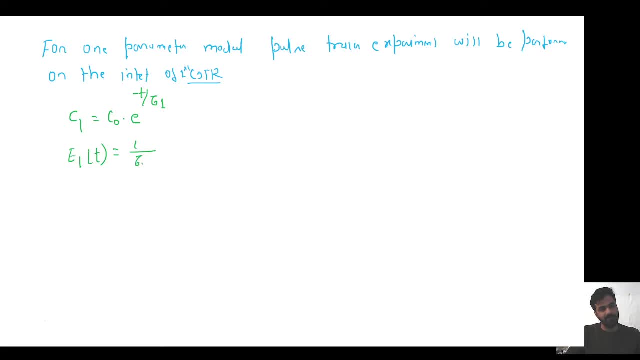 is RTD curve. that is equals to 1 upon tau i e to the power minus t by tau i that you know. this is the basic things in the CSTR and PFR continuous state tank reactor. this is concentration at the exit and this is the exit age distribution function. this is very important that you should. 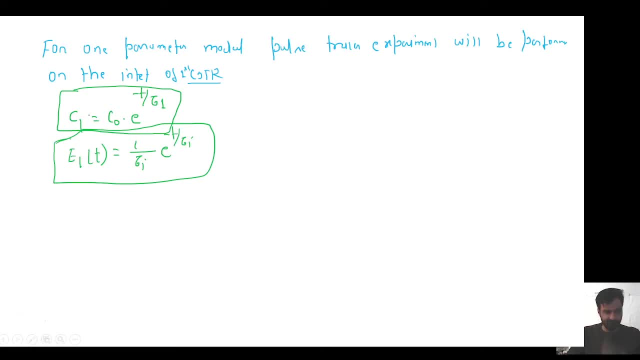 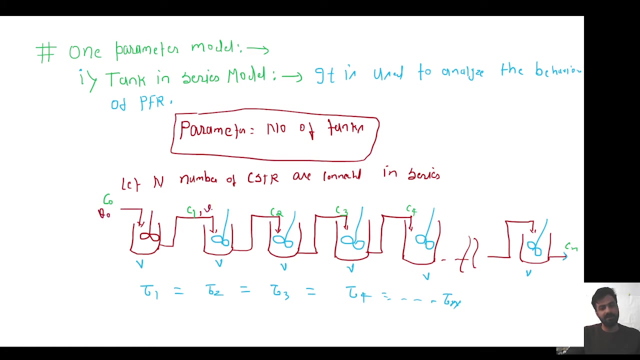 know. ok, now moving further, when we talk about you know I mean for second reactor. so can I write my decision C 1 into V naught? why? because here just try to understand, here I am considering volumetric flow rate will be same, so C 1 and here it is V naught. I am assuming mass balance over here. so 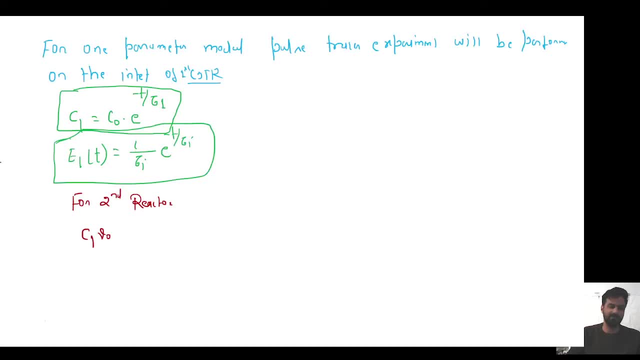 C 1 into V- naught. okay, that is mole balance. generally you can apply the mole balance in mass- C 1 into V naught. minus C 2 into V- naught. this is in minus, this is out. so you can write in minus out. plus generation, minus consumption, that is equals to. it is a rule. 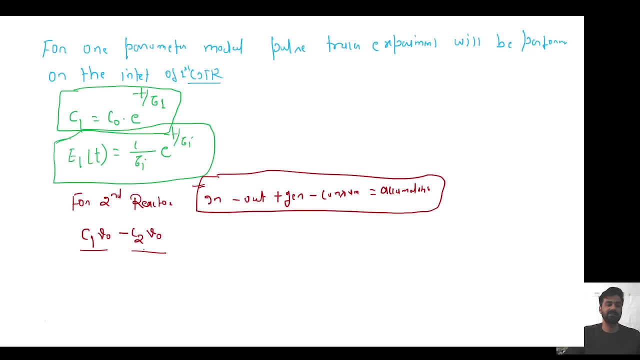 of thumb for any reactor of mass balance and mole balance of these things. so here, moles of address are in minus moles of dresser out. okay, there is no, any generation. you know, consumption of this things, that is equals to accumulation, that is equals to V and that is equals to DC, to upon. 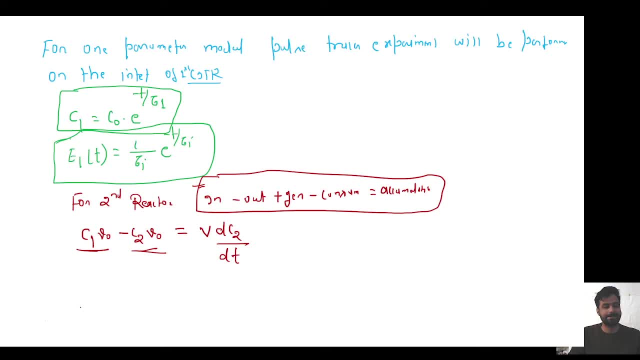 the DT at the exit of the reactor. are you getting? that is in, that is out and that is accumulation. okay, so C 1- you can write that is C naught- into e to the power minus t by tau 1 and n into v naught minus c2, v naught, that is equals to v, dc2 upon dt. are you getting so next? 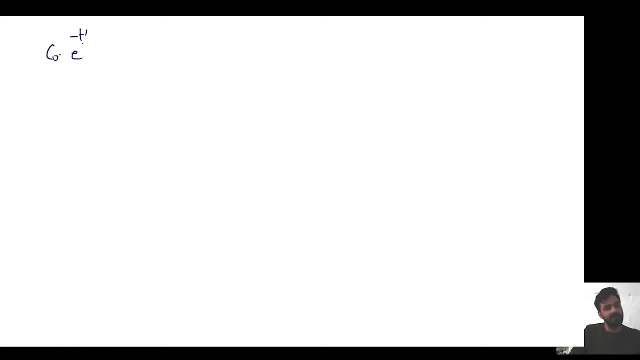 can i write c naught e to the power minus t by tau 1 minus c2, that is equals to v by v naught dc2 upon dt, why i have taken common v naught and after that i placed over here. can i write again c naught e to the power minus t by tau 1 minus c2, that is equals to: 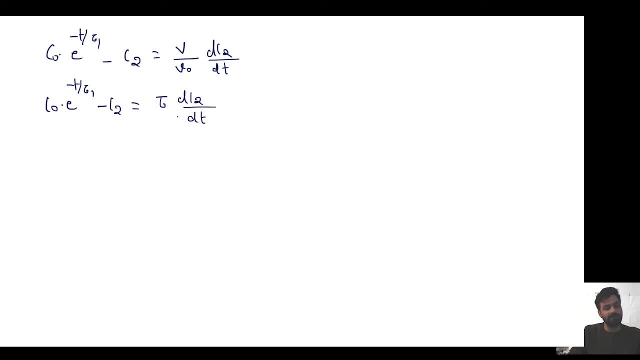 tau and dc2 upon dt generally. i am writing the tau i, okay, so can i write over here: c naught e to the power minus t by tau i upon tau i, okay. minus c2 by tau i, that is equals to dc2 by tau i. 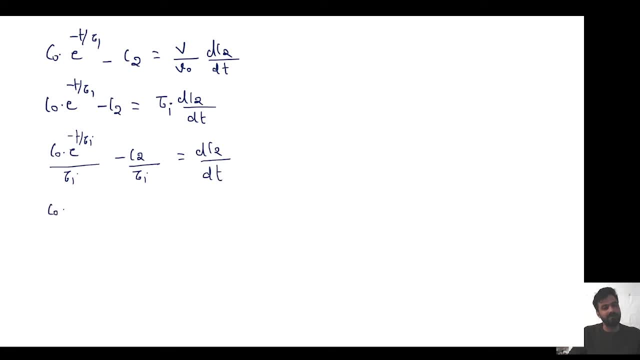 dc2 upon dt. so can i write c naught. i mean, can i write directly dc2 upon dt plus c2 by tau i minus c naught e to the power minus t by tau i upon tau i, that is equals to zero. so can you see, here this is a differential equation, this is a differential equation linear. 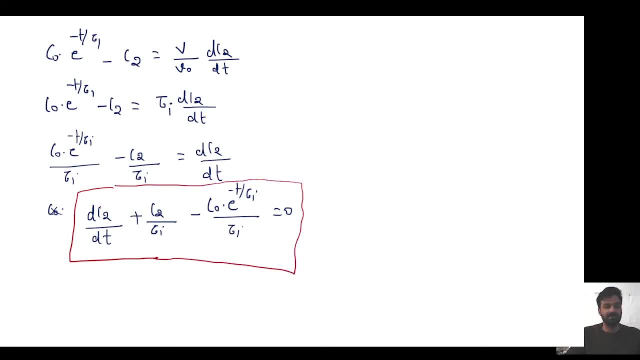 differential equation of constant coefficient. okay, so dc2 upon dt plus c2, tau by tau i. this is a linear differential equation. so we have to solve this differential equation and you all are very access in calculating this differential equation. it will be calculated by calculating integrating factor. 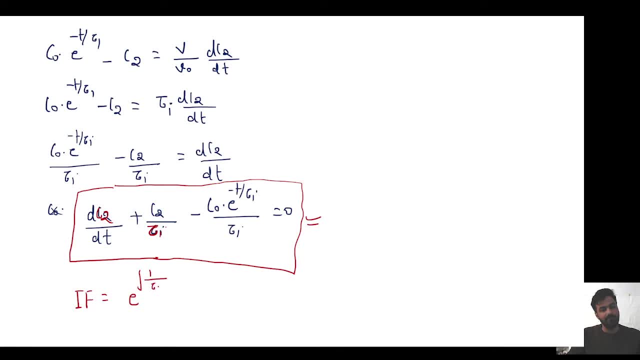 and it is equal to e to the power one upon tau i dt. so that is equal to e to the power t t upon tau i. so finally, you have calculated the, my dear friend, the integrating factor also. now the thing will be very easy for you. so once after, 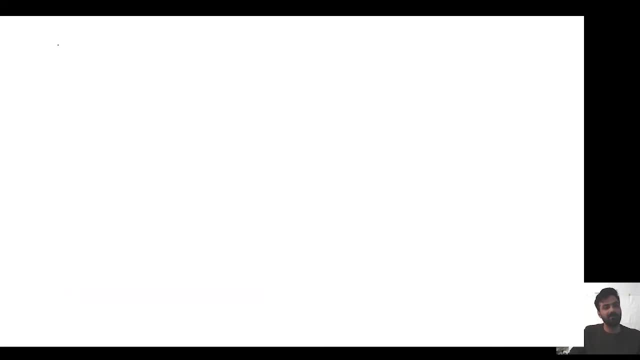 calculation: integrating factor. we will move forward to solve the problem. then I write c2 into integrating factor. that is equals to. I mean, if you are assuming this is in the form of this, that is equal to DC 2 upon DT plus C 2 upon tau i. that is equal to C naught t to the power minus t. 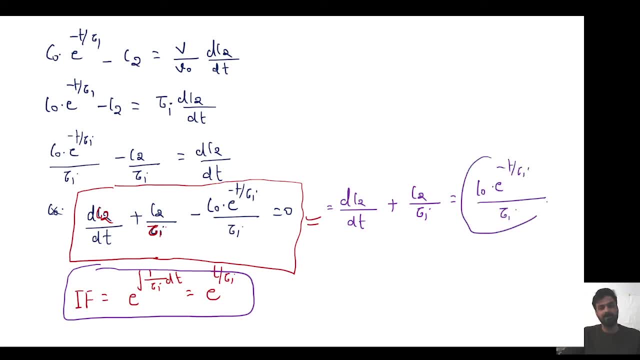 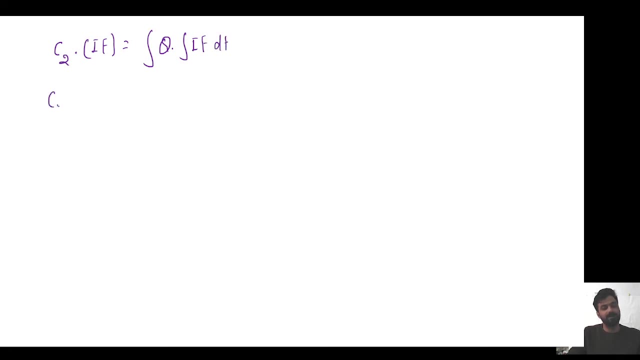 by tau i upon tau i. so if I am assuming this one as Q, okay, Q, that that is the general procedure of solving this differential equation. so can I write here: Q multiplied with integrating factor, and then it is equal to DT. so can I write again: C2 and integrating factor is equal to. 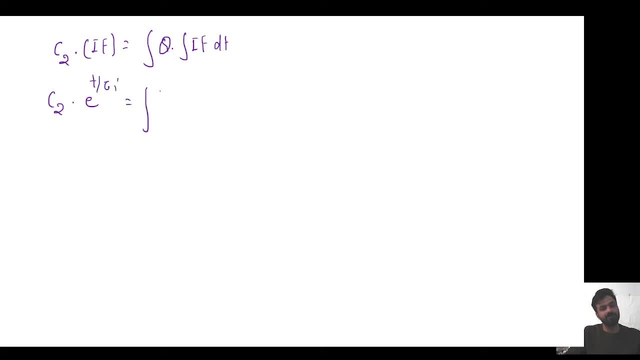 DT plus C2 upon DT plus C2 upon tau i, that is equal to C2 upon DT plus C2 upon tau i. that is the power t by tau i. that is equals to c. note e to the power minus t by tau i upon tau i. 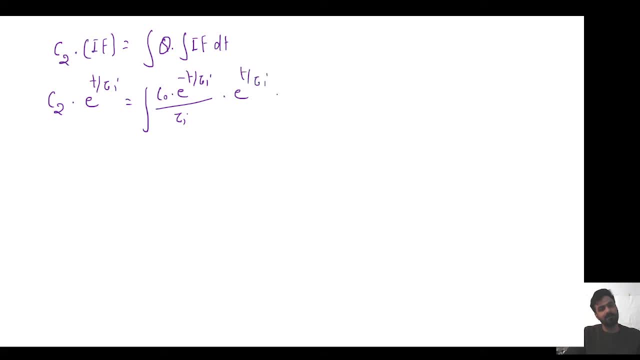 and e to the power t by tau i dt are you getting. so you can calculate this. you can write again c2, e to the power t by tau i. so once we do the calculation, so this is the tau i c note by tau i will get common. so it will be equals to c note and t upon tau i. plus you can write k. 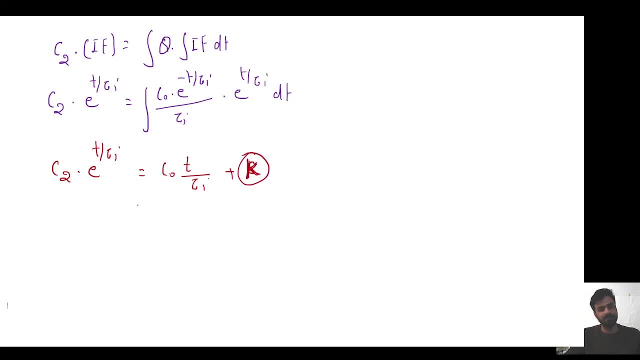 this is a constant, okay, so at t is equals to 0, c, note, is equals to 0. are you getting sorry? c2 is equals to 0. if c2 is equals to 0 and t is equals to 0, so k will be equals to. 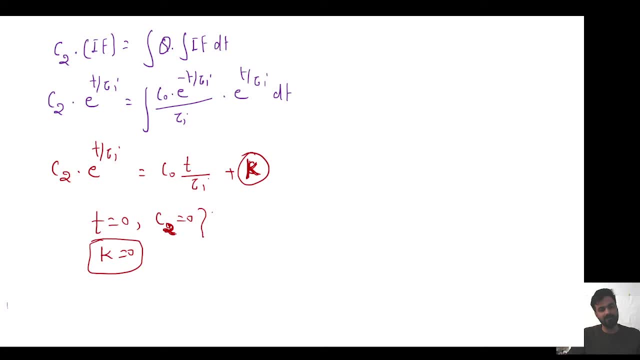 0. this is our boundary condition. so i mean no c2 will be there at. t is equals to 0. so can i write c2 e to the power? t by tau i? that is equals to c. note: t by tau i. are you getting so our? 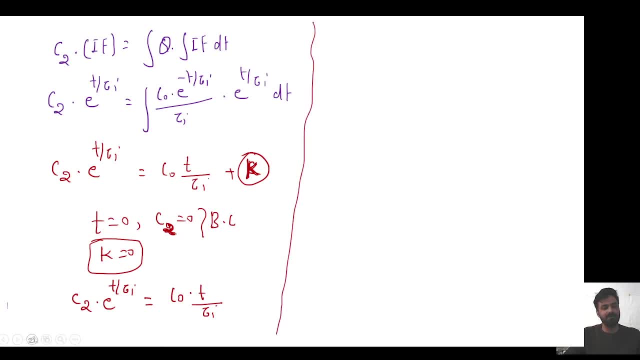 objective is calculate c2. okay, so our objective is to calculate c2. finally, you have got c2. this is the function of time. that is equals to c. note t by tau i. e to the power t by tau i. and if we multiply it with t by tau i, i am getting e to the power minus t by tau i i. 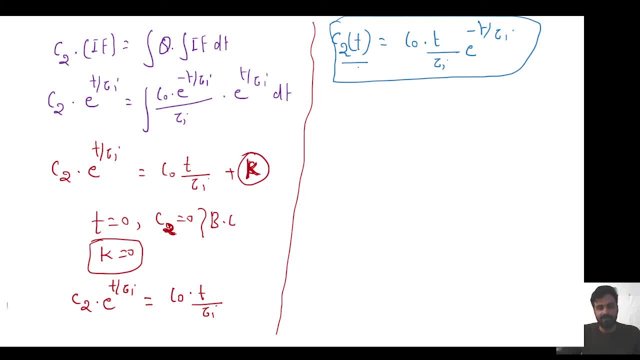 will get in c note t by tau i and e, a to the power minus t by tau i. so now you will have to understand the recurrence relation there in between. are you know the outlet, donation of every reactor? so i am writing the recurrence relation. so if you will write c3t you will be getting c note upon factorial. 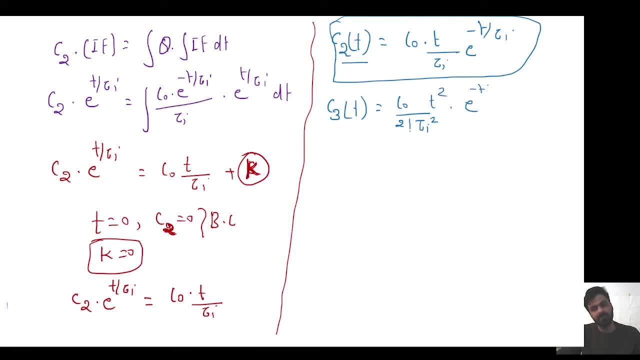 two tau i square, divided by between tau i plus out tends to zero, is equal to tau i squared and d b sacred to the y circle. the power is equal to e to the power minus t by tau i minus t square, e to the power minus t by tau i. So you can understand there is a recurrence. 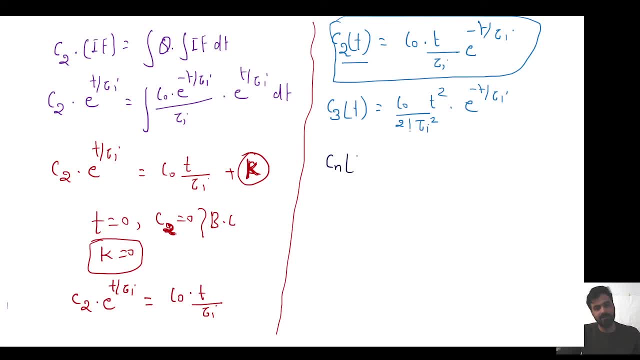 relation that you can see over here. So I am writing directly: c n t. c n t, that is equal to c naught ok upon t by tau i whole to the power n. And here you can see if here it is 3, here there is a factorial of 2 means 3 minus 1 factorial. So here you can write: 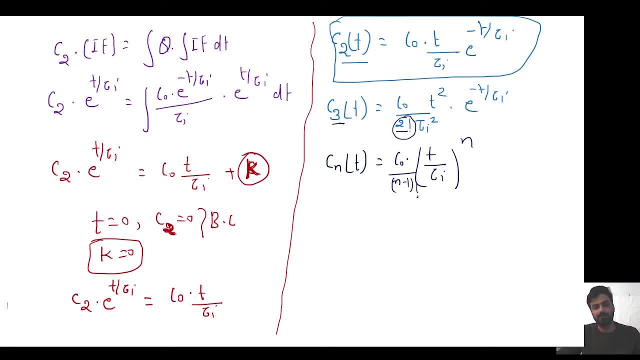 n minus 1 factorial. Are you getting Here? there is a n minus 1 factorial, It is factorial sign. ok, I am writing over here. And e to the power minus t by tau. i Again I am writing here. that is c n t. that is equal to c, naught upon n minus 1 factorial. And here you can. 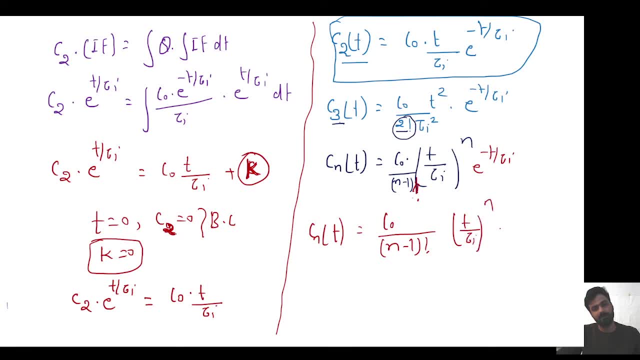 see, there is a recurrence relation that you can see over here. So I am writing here: c n, t by tau i, whole to the power n, e to the power minus of t by tau i. ok, So this is the recurrence relation and you can calculate the concentration at the exit of any particular. 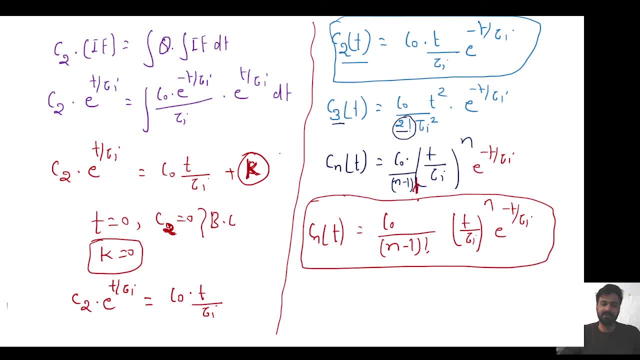 react. Are you getting So, my dear student? you can see, at t is equals to n, at t is equals to 0.. At t is equals to 0, concentration will be 0 and t is equals to infinity. again it. 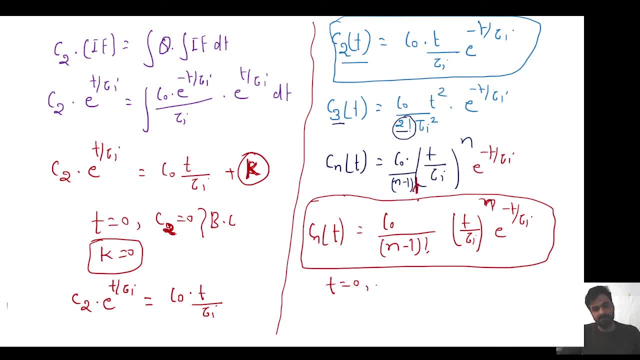 will be 0.. Are you getting So? at t is equals to 0, c n. t is equal to c. naught upon n minus 1 factorial c n is equals to 0 and at t is equals to infinity. again, c n is equals. 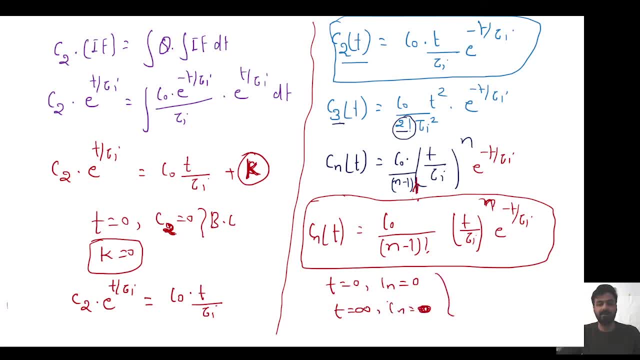 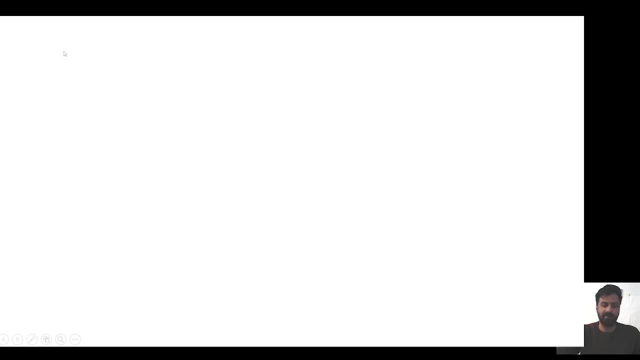 to 0.. So I mean there, definitely there must be a. I mean the curve will be increasing and again decreasing. There must be a maxima, ok. So I mean you can calculate the thing from here. The plot will be like that. The plot will be like that If here it is c t. 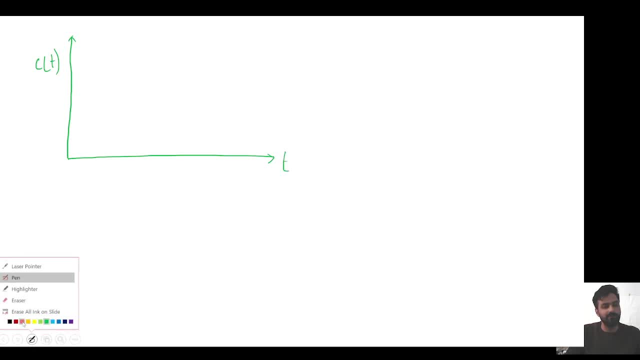 it is equal to n plus time, so the plot will vary in this way: it will be 0 initially, it will go to maxima and again it will come to 0.. Are you getting? So? this is the concentration versus time curve for n cstr. ok, Now, when we talk about my dear student e t, ok, E. 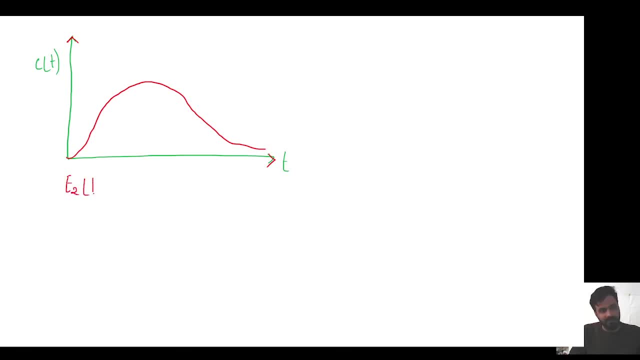 2t e 1t. we have calculated, So can I write, president, e to the power t over e sub delta. ok, minus t upon tau i divided by t and multiplied with e to the power minus t by tau i minus. 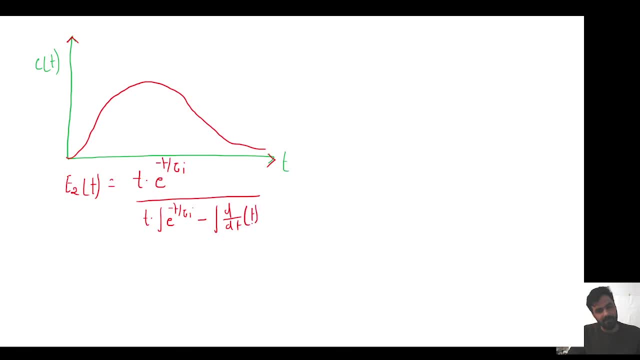 d upon dt of t and again e to the power minus t by tau i. it's as simple as that. this is just an integration, okay, so finally you will be getting t upon tau i square and e to the power minus t by tau i, e to the power minus t by tau i, so finally you can calculate e3t also. 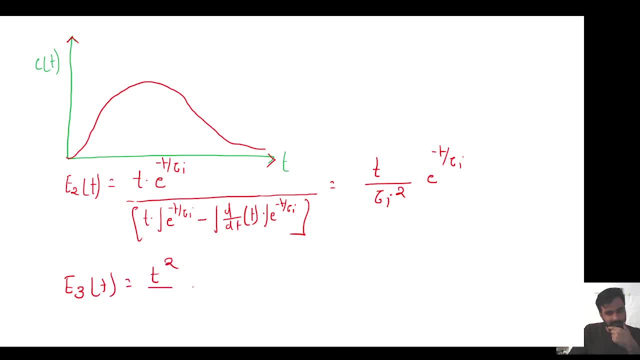 and that is equal to t. square upon tau, iq and factorial 2, okay, and e to the power minus t by tau i. that you don't need to derive everything here. i am deriving to let you know. so again you can see there is something uh related to this one. 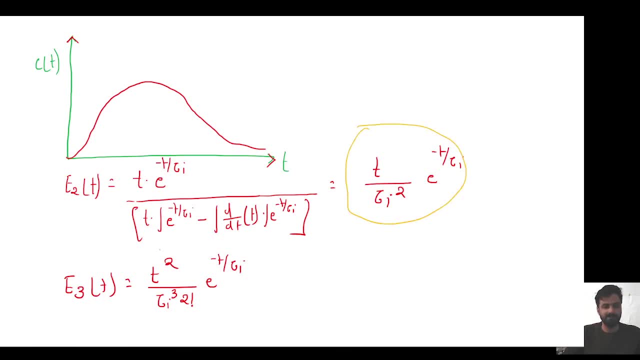 and this one. so you can see there is an expectation of the recurrence relation. so i am writing here the recurrence relation so directly. i am writing e and t. that is equal to my addition t to the power n minus 1 upon tau i, equal to power n. 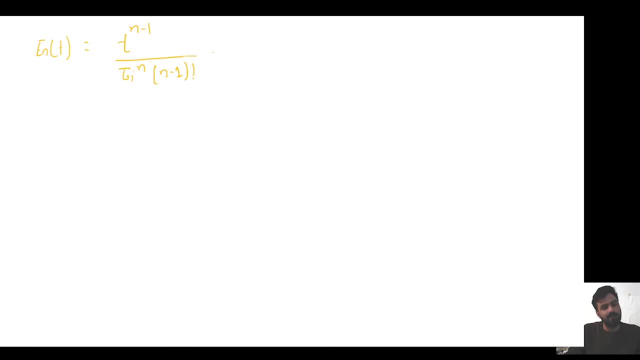 n minus 1 factorial, and e to the course minus e to the power minus at toˡ T by tau I. Are you getting A to the power minus T by tau I? So here this is the recurrence relation of this particular thing. Okay, For RTD function. This is our RTD function of. 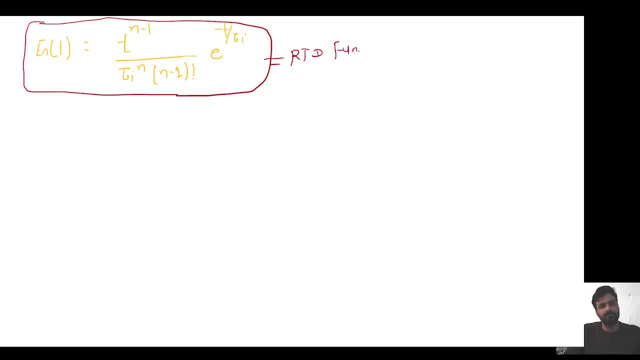 N-th order. N-th order: reactor in series: RTD function. Are you getting? So we have calculated, you have derived the RTD function. now. Now try to understand one thing, I guess, and what is happening? The mechanism is very important over here. I am letting you to know with the 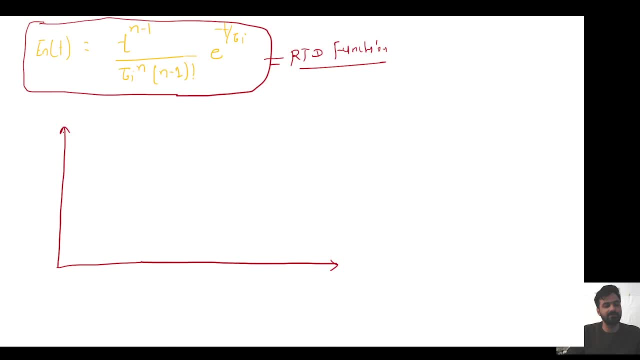 help of the graph, then it will be very easy to visualize you. So if I am telling you it is ET and if it is T plot, If it is ET and if it is T plot. So finally, when N is equals to 1, the plot will varying like this You can see. 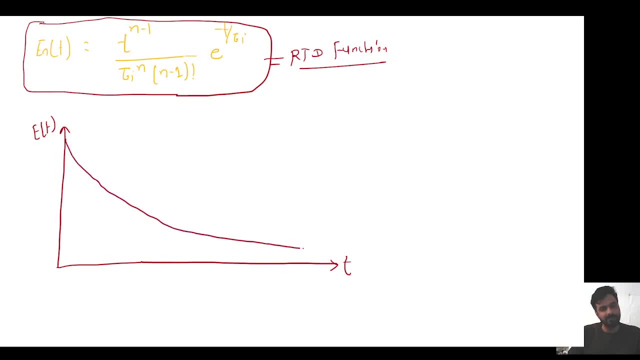 The plot is going like this: ET versus T graph: Are you getting: When N is equals to 1.. When N is equals to 2. The plot will be coming like this: There is a broad plot like this And again it will be going like this When here I am writing: when N is equals to 1.. When 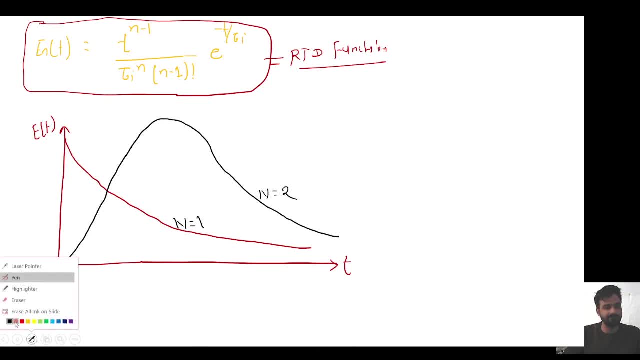 N is equals to 2.. Are you getting Again? I am telling you: when N is equals to 3, It will go like this. Again, I am telling you this: it is when n equals to 3. again, I am writing this plot- is when n is equals to 4. 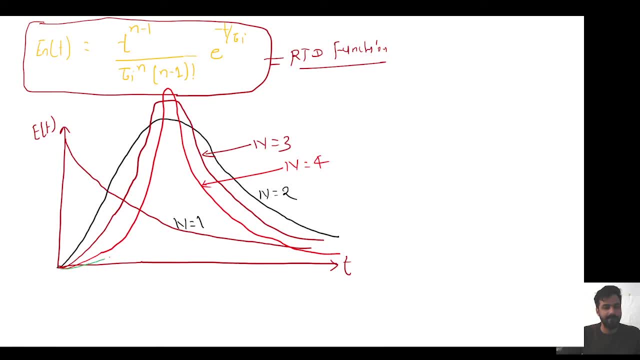 okay, green is when n is equals to 5. okay, and you can see there will be a plot like this one when n is equals to infinity. so when we talk about ET curve of PFR, ET versus T curve of it, is PFR how it look. 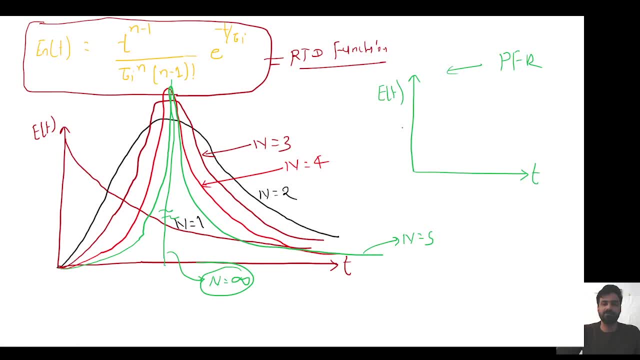 like you. just try to understand. it used to be. look like this one. it is a direct delta function. and again, here you also see when n is equals to infinity, when n is equals to infinity, it also looks like this. so the plot will be like this. so can I say here from the plot, when n, CSTR having equal volume? 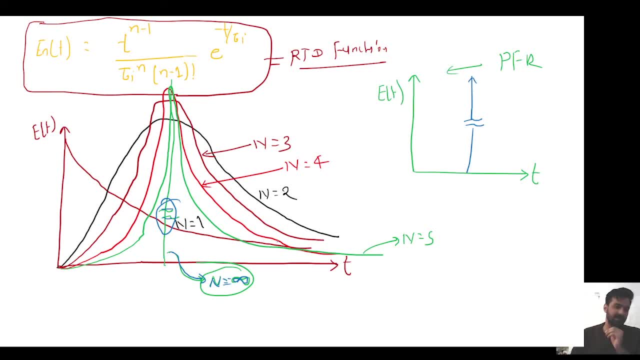 connected in series will work like a single PFR, are you getting? so? this is the objective of this session, that how this n CSTR having same volume when we are connecting it in the series, then they will work as a another PFR. okay, so this was the objective of this thing, so hope I have tried my best to let you. 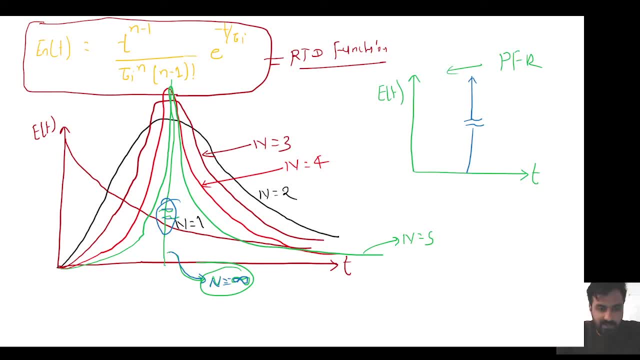 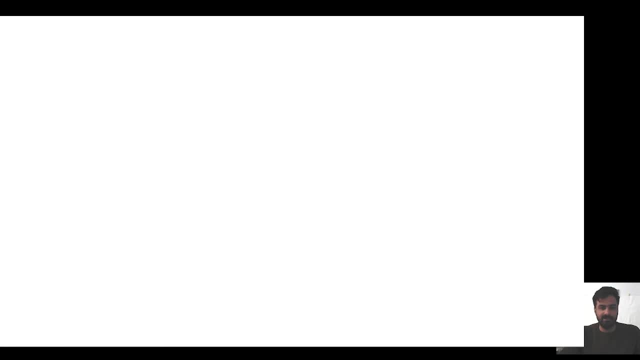 understand your thing, how this things work like that, okay. so I think up to this, everyone is very clear: all of the thing that I have late minister in the tank in series model and how we can derive the thing, how we can calculate the- you know- concentration at 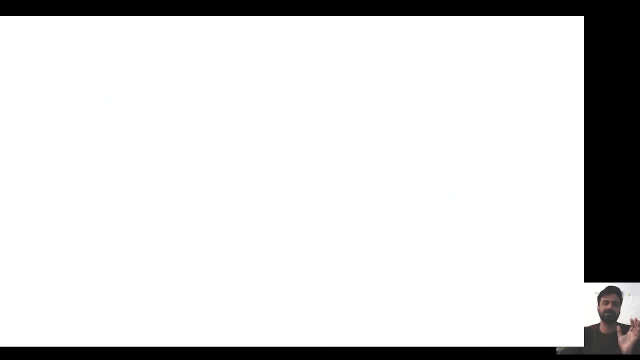 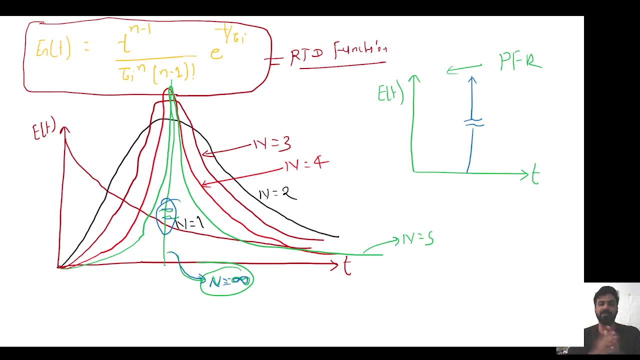 the exit of any reactor, how we can calculate the R TD function at the exit of any reactor and how the number of series and CSTR connected in series will work like a PFR graphically. okay, so in the next section lecture I will be discussing how we can calculate the number of times and how we can calculate the. 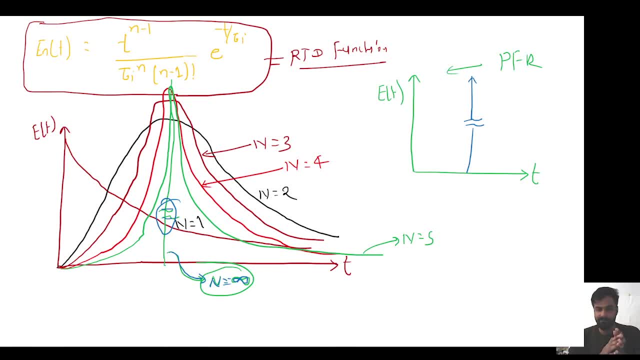 conversion from n CSTR connected in series. okay, so thank you for all. thank you for watching this video and if you are facing any doubt, you just you know, go through this video and it will you let you get to know how we can solve the problem on the basis of this concept and at the end of 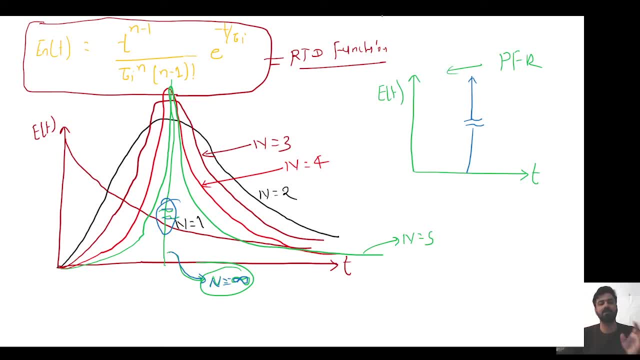 this session, when I will be completing the one parameter model, I will, you know, solve some numerical problems, so from there you can get a good idea how we can solve the numerical from this particular concept. okay, so thank you all.